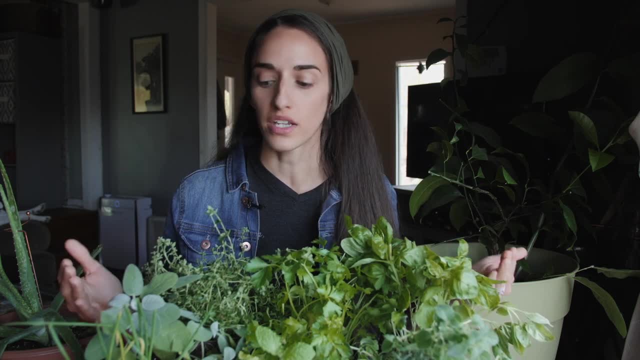 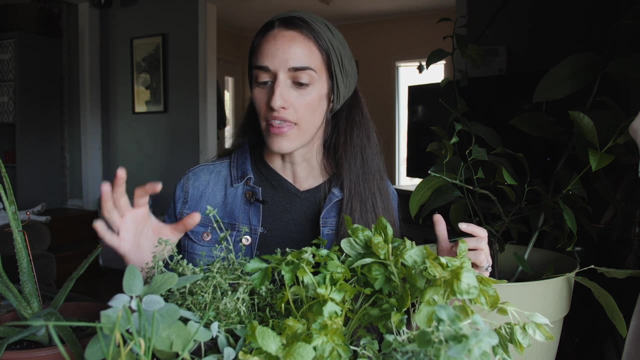 affect your outdoor gardening. But in terms of outdoor gardening, your zone that you live in is going to matter, And when gardeners talk about zones, it's basically just your climate And that zone. certain things will thrive and certain things will not do as well. So it's good for you to. 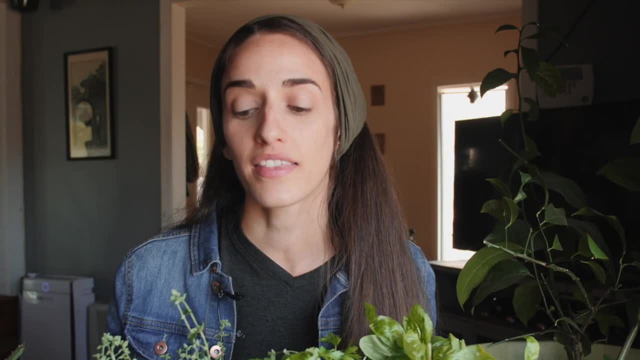 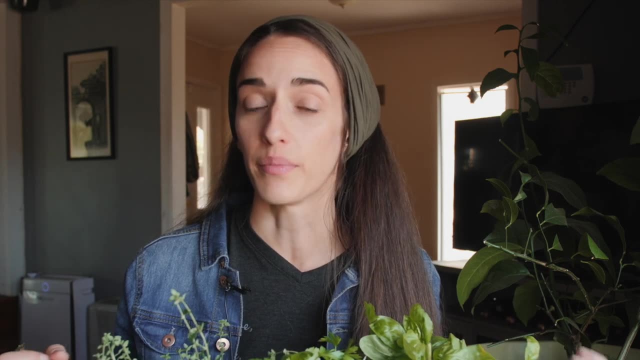 figure out which zone that you are living in. Another great thing about herbs is that they are versatile in terms of how you can grow them. You can grow them in pots, you could grow them in a windowsill, you could grow them indoors, you could grow them outdoors. Some of these herbs will do better in full, direct sun, and some herbs will do better in part sun, And some herbs will even tolerate a decent amount of shade. Some herbs will also be contained to smaller areas, and some herbs in terms of lemon, balm and mint, things like that, they're going to want to. 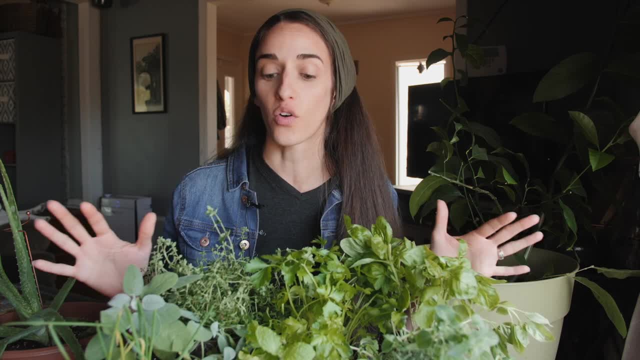 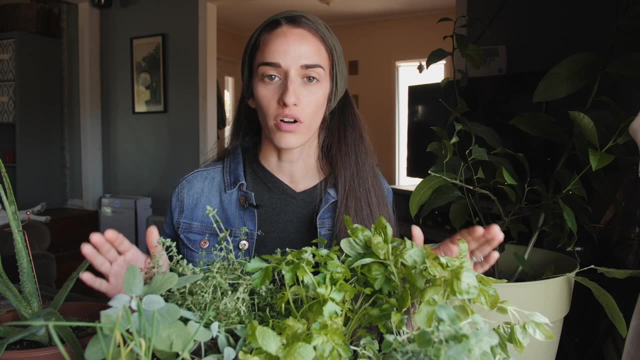 spread. So if you're going to put those in certain areas, they will take over their zone. they like to claim their territory. But again, do not get overwhelmed. Pick four or five hardy herbs that will do better in full direct sun, and some herbs will do better in part sun, and some herbs will even. 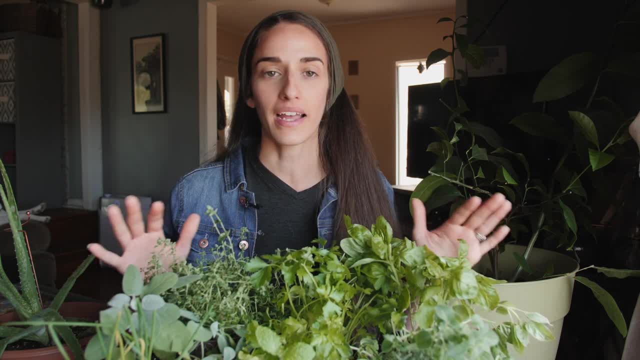 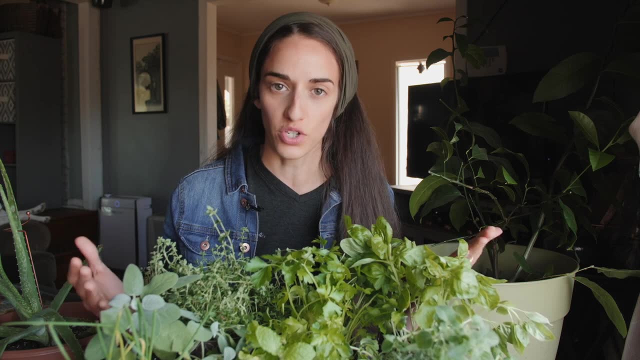 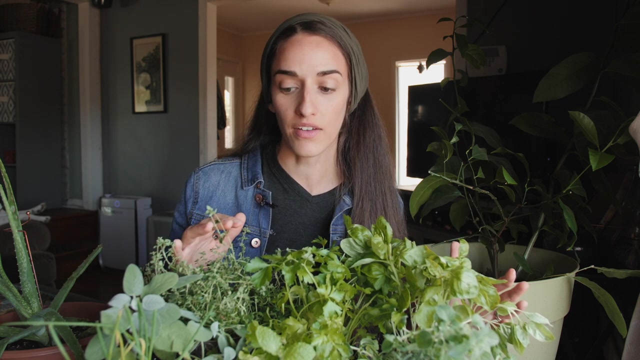 kill And just pick a nice sunny spot with filtered light. We are going to get through this. That's another thing that I usually recommend to people is start with the hardier perennial herbs. Some herbs are going to be more tolerant of things than other herbs are, And I'm going to go over the 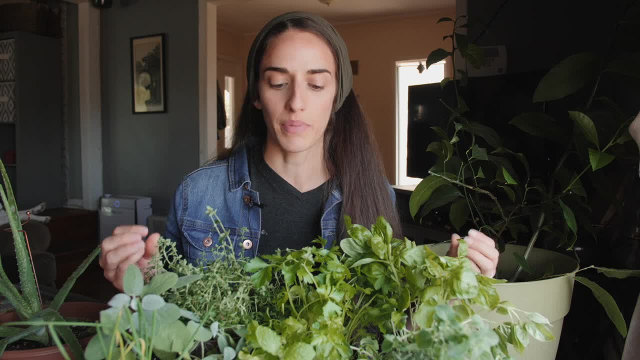 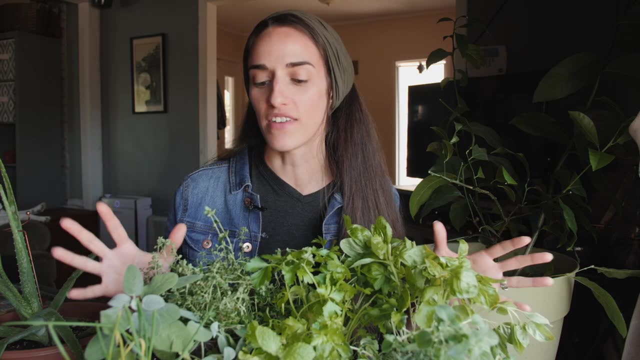 basics of that today. But that's my recommendation is: pick out four or five very hardy herbs that are hard to kill So you can get your confidence going, and then maybe you can venture out into some other types and species of plants. And I'm telling 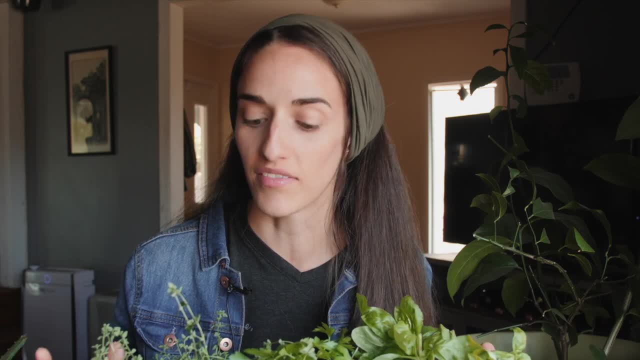 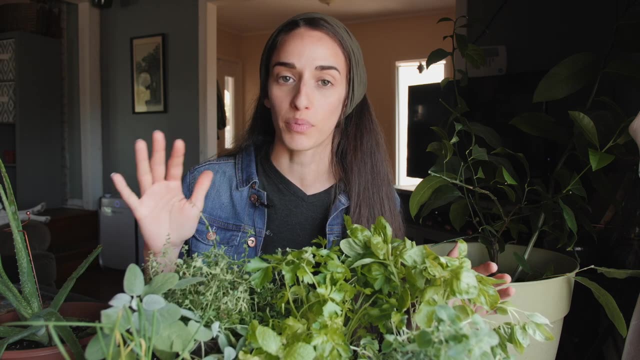 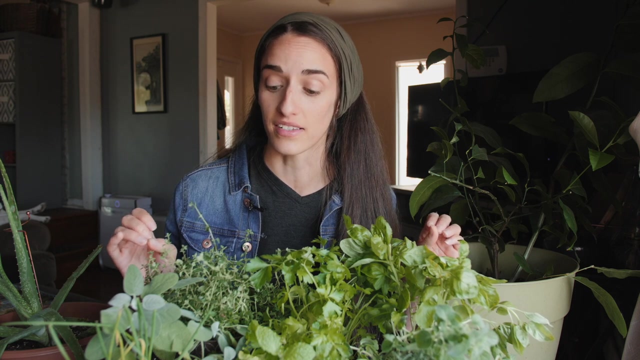 you. the world of herbs is amazing. You're going to love it once you get into it. And another great thing is that even within one simple type of herb like thyme, there are multiple varieties. With mint, there are multiple varieties. There's even a chocolate mint- Oh, yes, there is. And there's lemon. 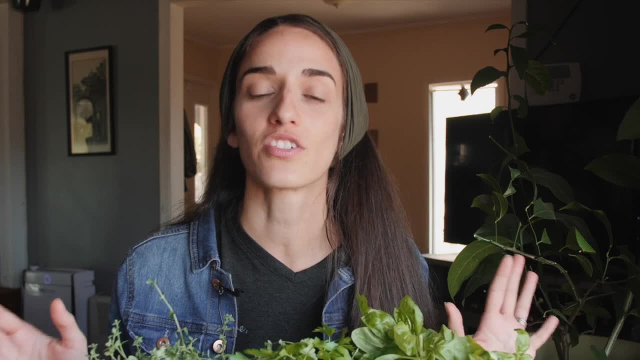 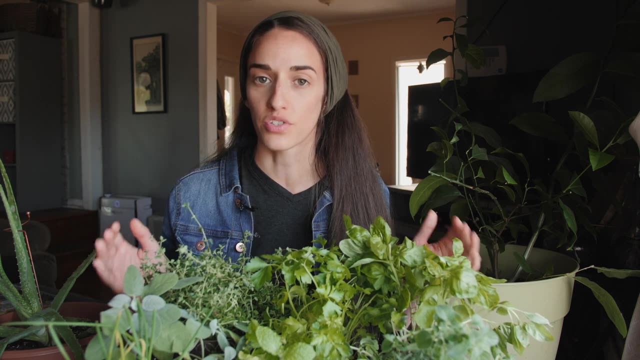 thyme and lemon, mint and things that make a lot of difference. So if you're looking for something that's going to make the whole world smell just a little bit better. So again, some of this information will change and be varied based on your zone and based on the type of soil you have, But there are. 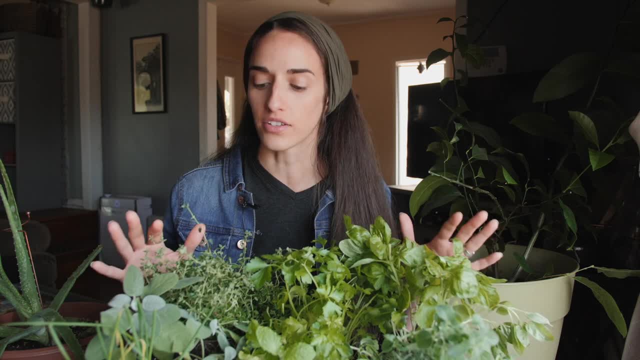 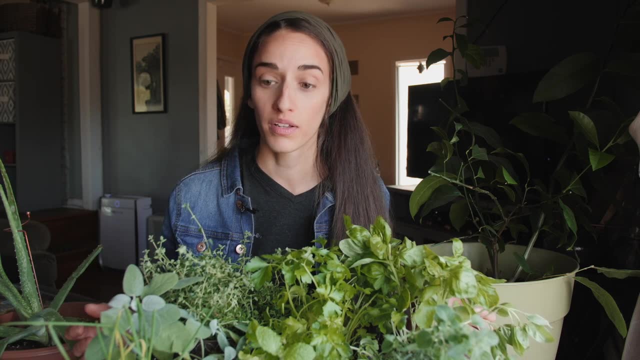 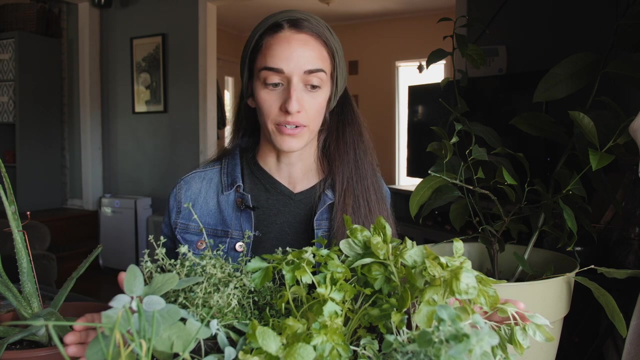 certain herbs that I have found are tolerant to many different types of environments. All right, so we're going to get into the basics. Let's recap: You got to have hope. There are hardy breeds of herbs that are very hard to kill, And it will make your life smell a little bit better. 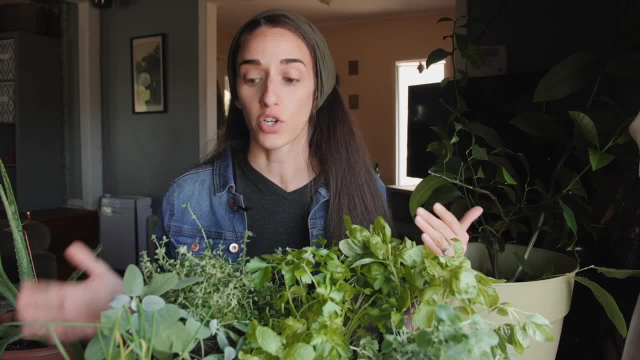 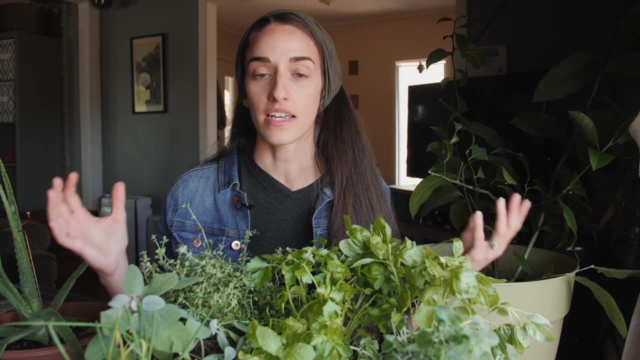 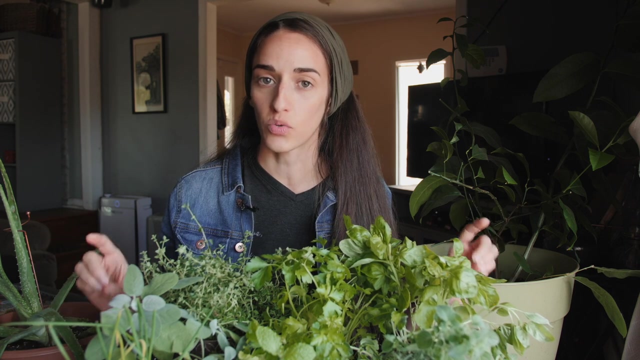 So there are perennial herbs and there are annual herbs. Perennial herbs are herbs that are going to come back on their own every single year, so long as the environment is nurturing to them. Annual herbs are ones that you have to replant every year. However, some annual plants will self-seed. 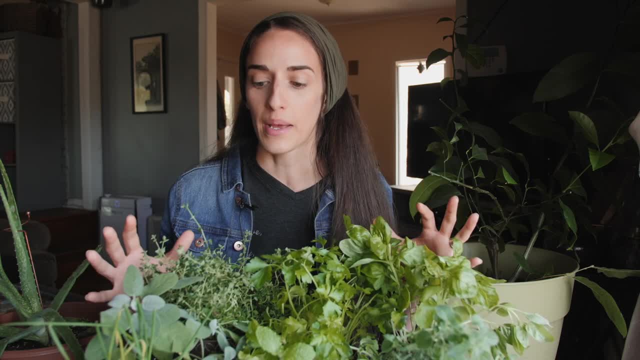 I really like to grow perennials because each year it's like a little surprise to see that plant come back and it brings a little bit of a change. So I'm going to show you how to replant perennial herbs. So there are perennial herbs and there are annual herbs. Perennial herbs are herbs that are going to 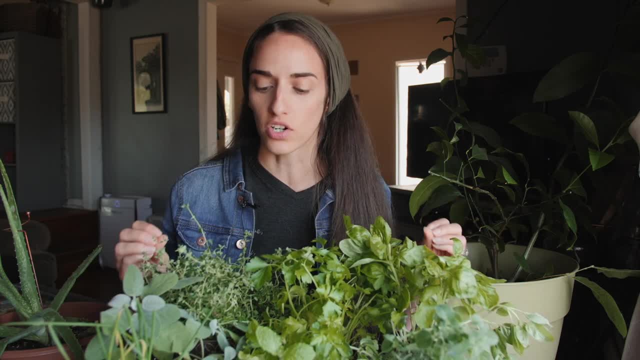 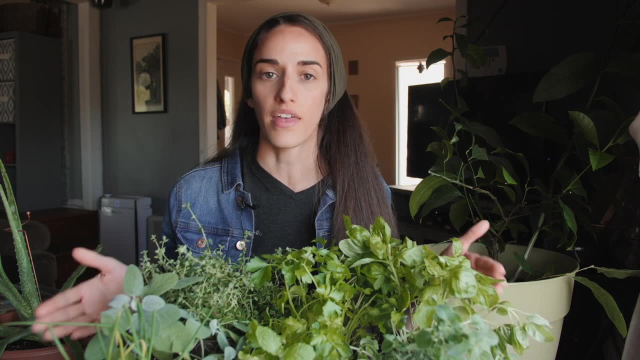 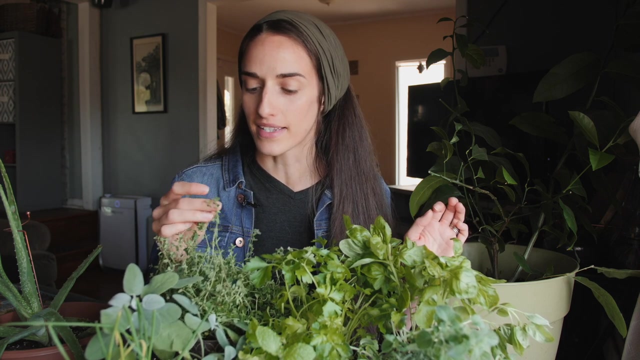 bring a little bit of joy to my heart, And I also find that the perennial herbs tend to- not in all cases, but tend to be a little bit more tolerant and more hardy than the annual herbs. So some of my favorite essential hardy herbs- number one: I got to talk about this guy because it's right in. 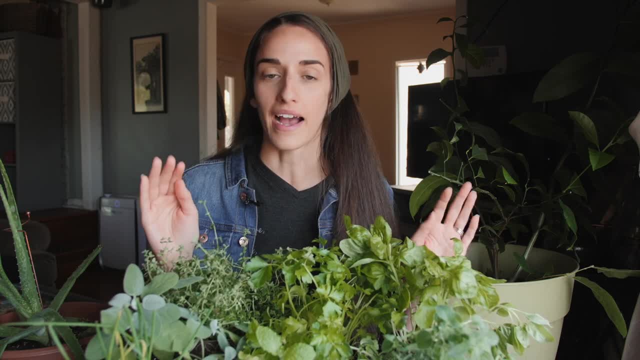 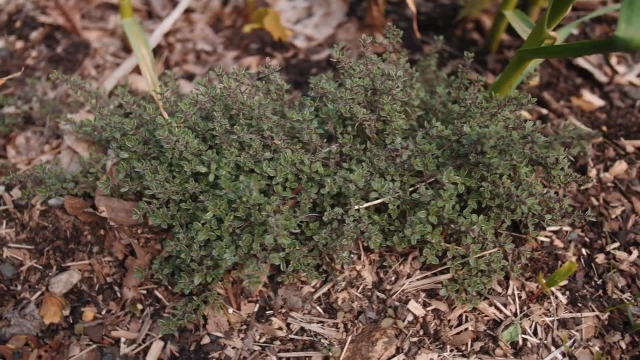 my face and it's smelling real good is thyme. I actually have a few bushels of thyme out in one of the front raised beds. It's silver thyme, Very beautiful, And it lasted all throughout the winter and is now waking up again, But it looked beautiful throughout December. 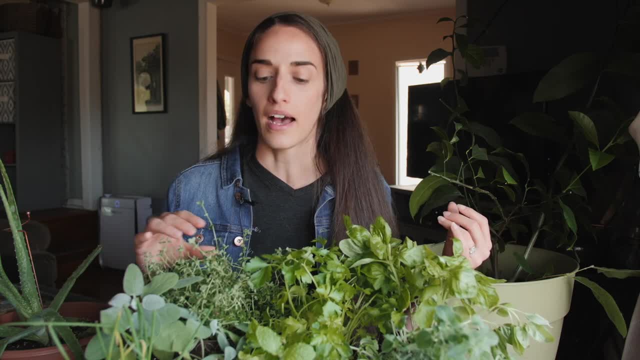 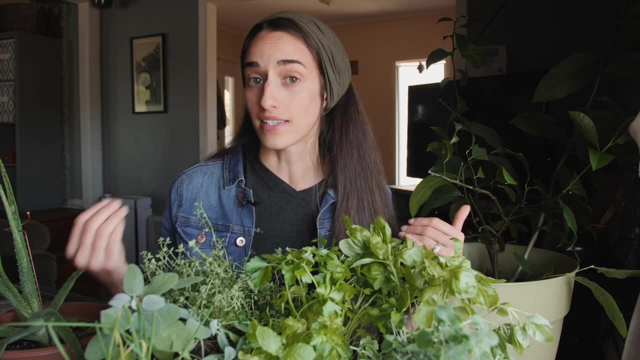 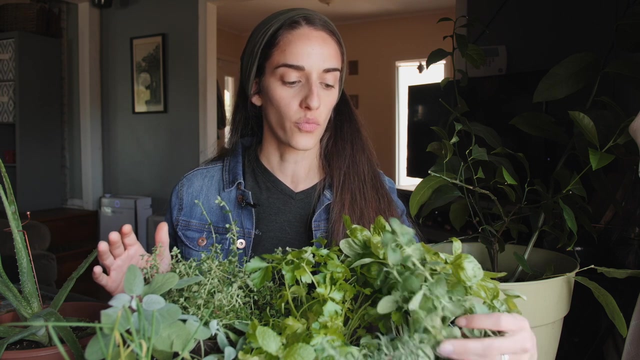 January, February, all the way leading up into spring Again. it is a hardy, tolerant herb that can be used medicinally. It can be used as a tea and it can also be used as a culinary herb. Another hardy herb is oregano. I have that up here in the front Again. 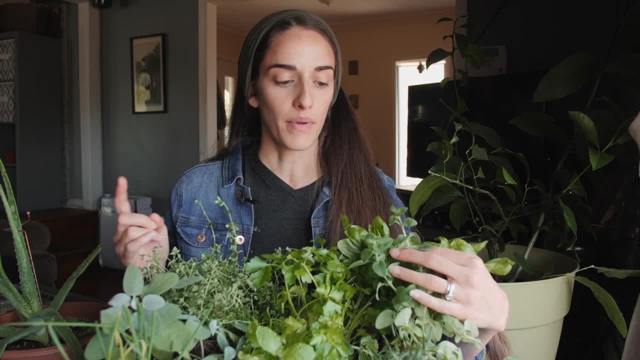 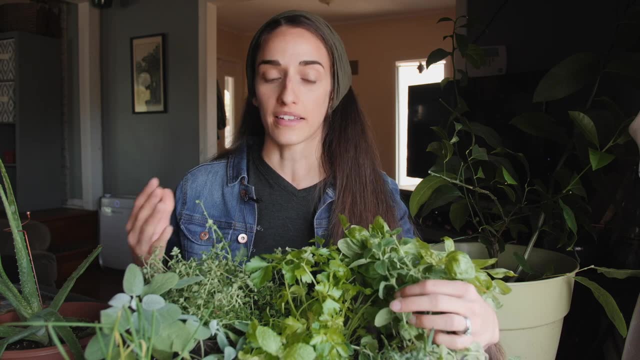 there are different types of varieties of oregano, but that's a different type of herb. That is one that will come up by itself every year. I planted some in my dad's garden last year and it lasted pretty well through the winter, and now it's starting to grow again, So another. 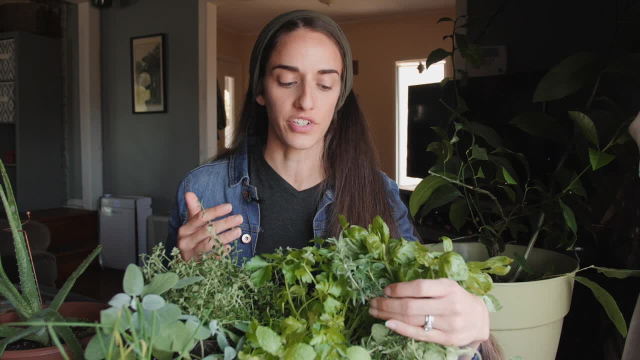 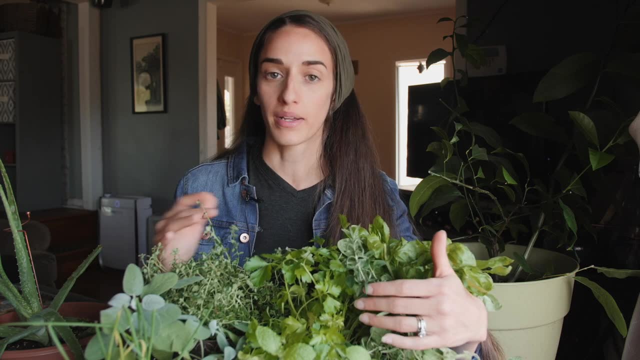 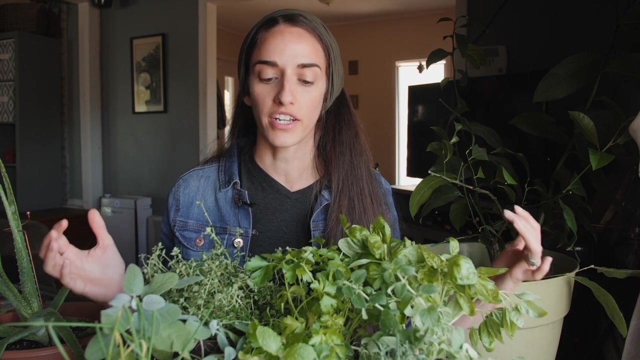 hardy herb that is perennial, that will come back year after year and in some climates again will survive all winter, is rosemary, Another herb that I love to use in a lot of cooking and is also medicinal in nature. And of course, I can't talk about hardy herbs without 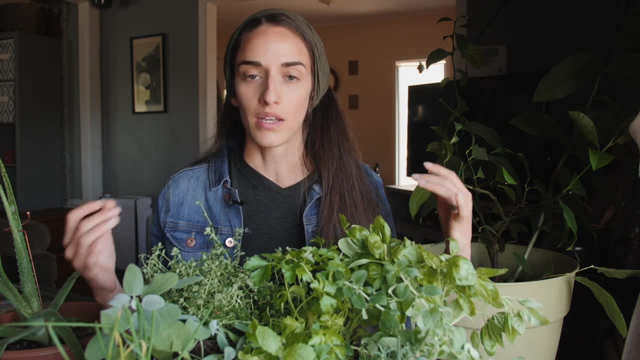 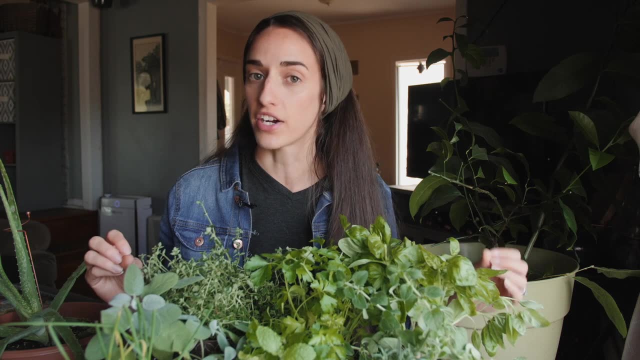 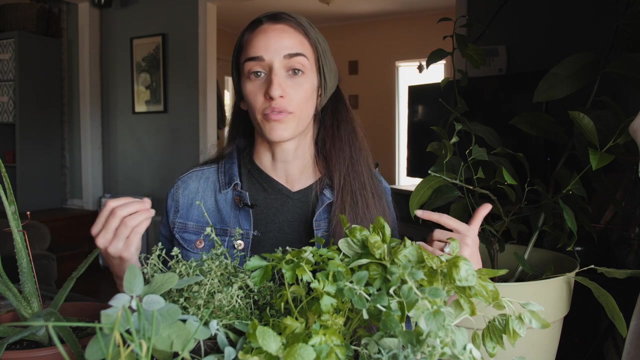 talking about mint and lemon balm. Mint and lemon balm are very prolific. They will take over an area. They tend to be very hardy and very tolerant and very easy to grow. They are wonderful in iced teas, They are wonderful in drinks, They are wonderful in food. They are wonderful in salad. 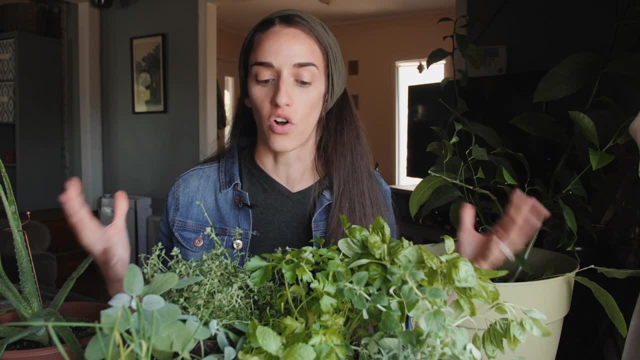 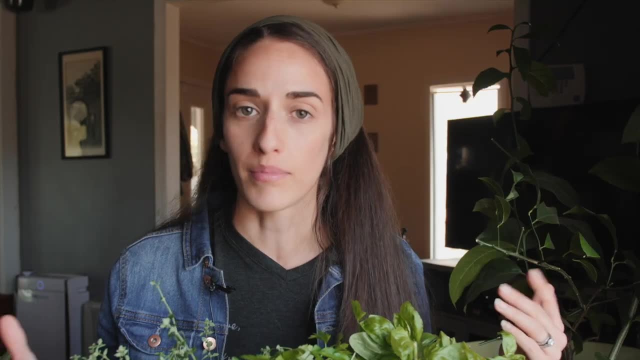 They also have medicinal benefits. You can make them into teas and tinctures and all of that wonderful stuff. They will also help prevent pests and certain bugs in an area. Lemon balm is one of my favorite teas. It's antiviral and it is wonderful. My lemon balm last year grew. 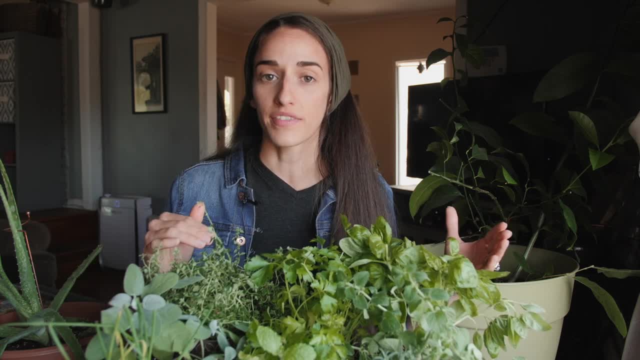 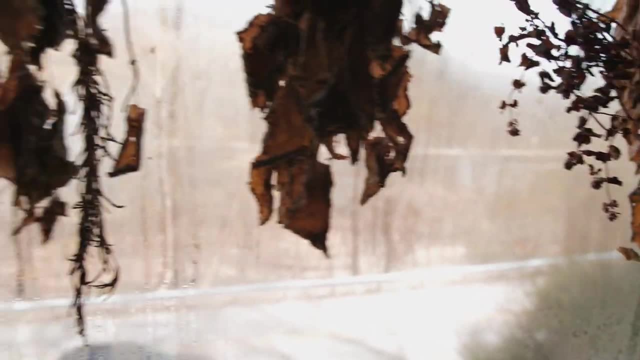 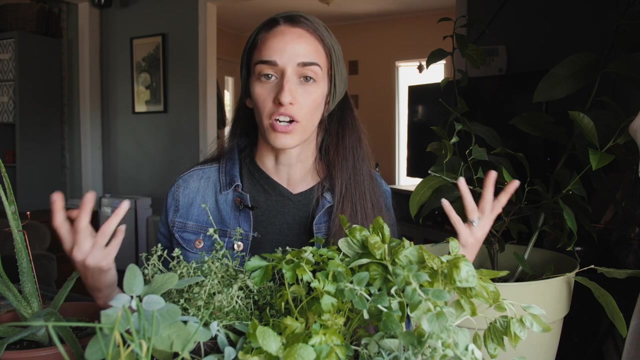 all the way into November and that's when I harvested it, dried it and hung it in the window. I have a bunch of herbs drying in the window that I am about to grind up now, as we're getting into the season where we will have a lot of new herbs to grow and harvest. We like to give herbs to our 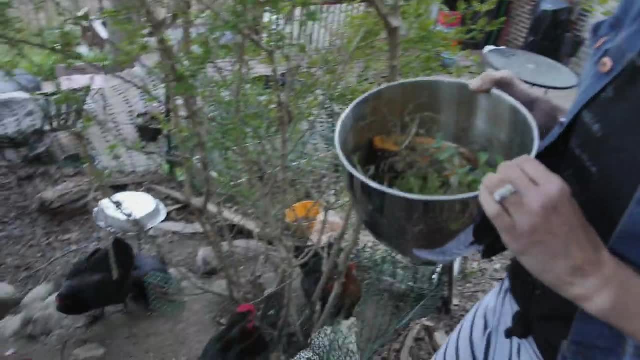 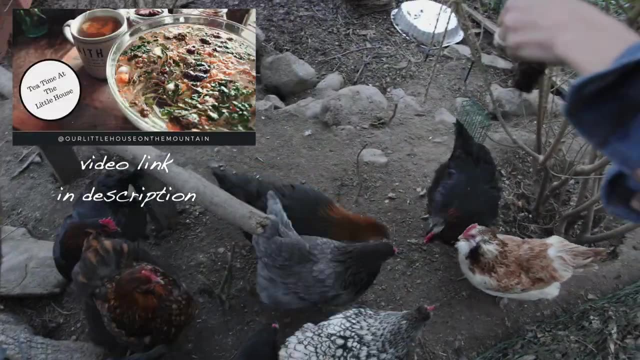 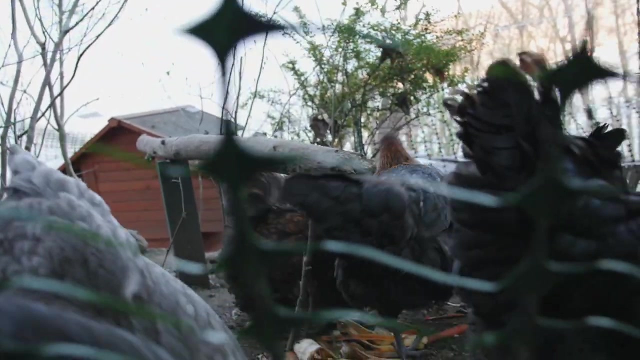 chickens. Herbs are wonderful for the health of most livestock and for the chicks. I give them herbal tea, I put it in their salads, I hang it from areas in their coop and it's just a wonderful immune booster, not only for them but also for us. Herbs are very 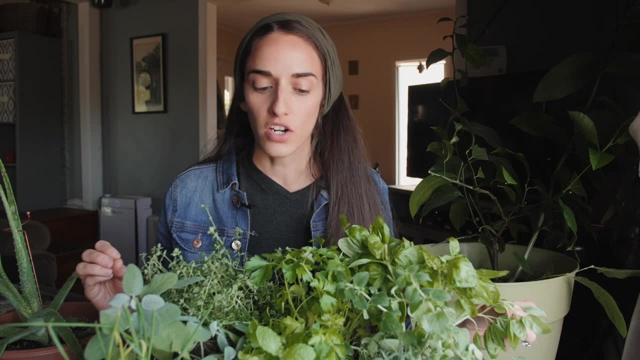 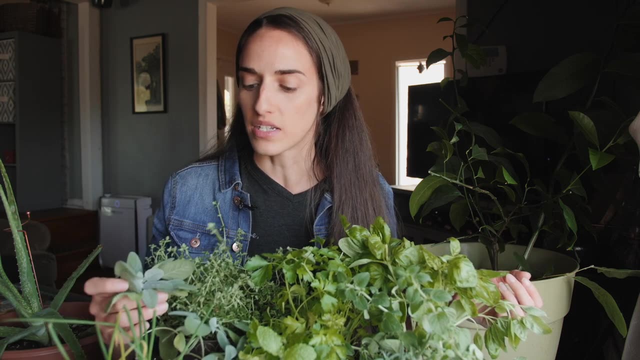 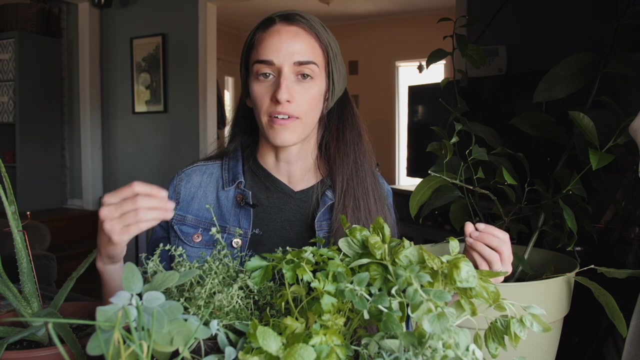 nourishing and healing for the body. Some of the herbs that I would say fall in the middle in terms of being hardy and a little bit less hardy. One is going to be sage Again. another beautiful culinary herb: Parsley. There are two different varieties I find. 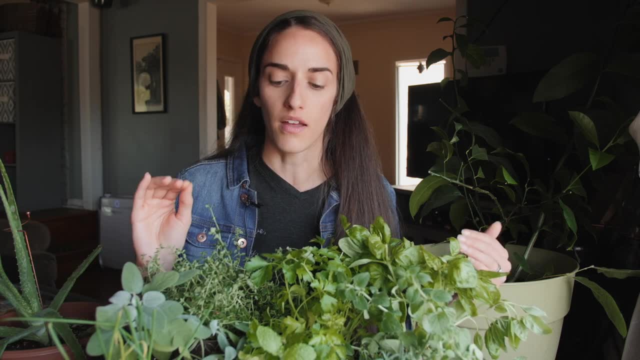 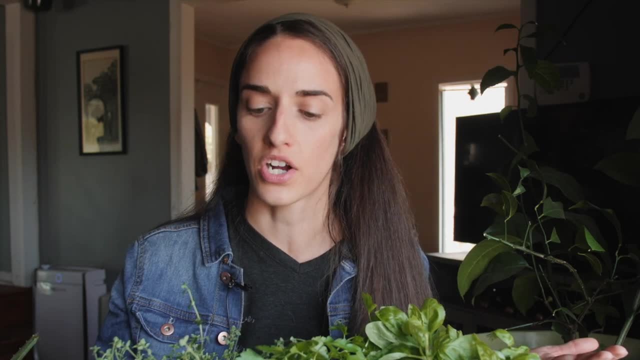 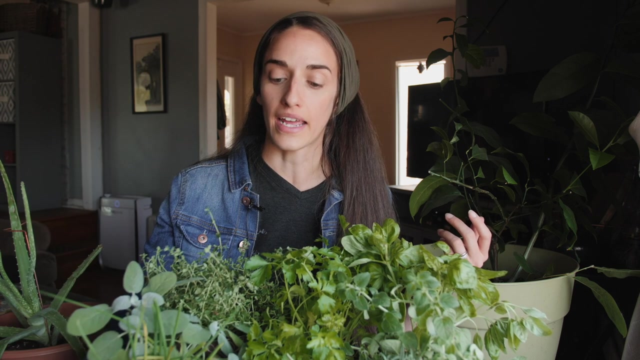 that the curly parsley is a little bit more hardy than flat parsley. Another herb that is in between, in my opinion, hardy and a little bit less hardy, is chives. Chives are wonderful in everything: Dried in cream cheese, put in soups, put in eggs. Delicious That's always. 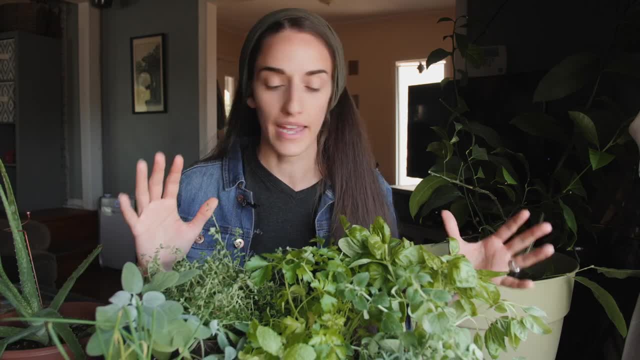 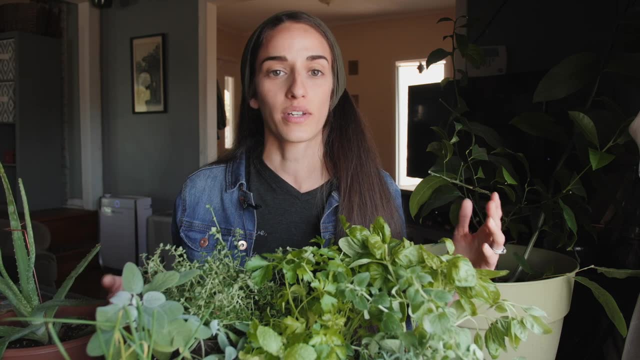 one that I like to have growing around in lots of different places, And aloe. I have some aloe over here on the side. Aloe can technically be considered an herb, and I always like to have it in different places. I like to have it in different places. 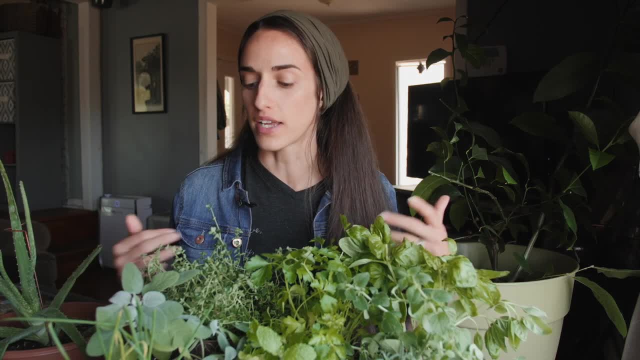 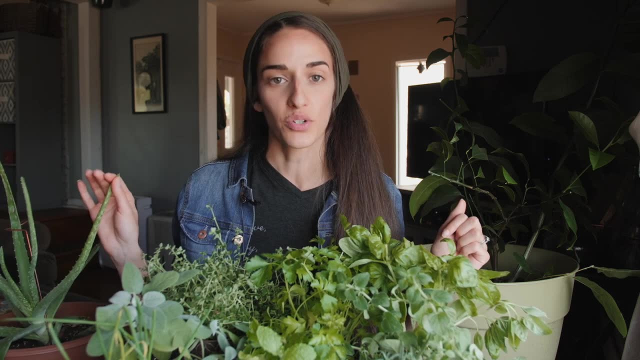 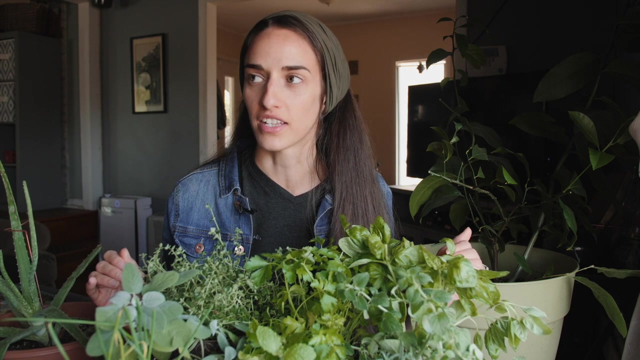 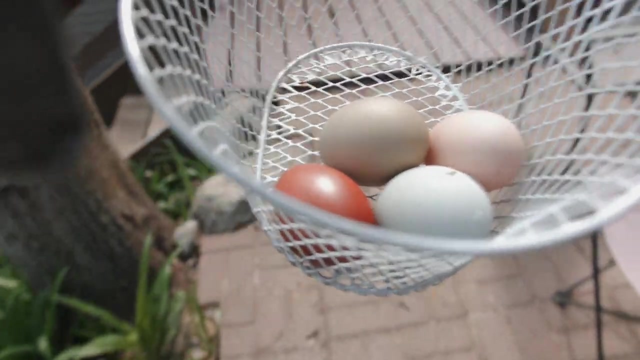 I always like to have aloe growing around. It's great for burns and all types of different skin issues. So aloe is always growing in my kitchen and I have two big plants of it right now in the dining room. Now the two herbs that I love to use is a chicken laying an egg. I've had chicken laying eggs for about a year and a half now. I'm trying to find them that way Now, the two herbs that I love to use in the summer, but they are a little bit less tolerant. Again, this would depend on your climate and the zone you're in, the type of soil you have. 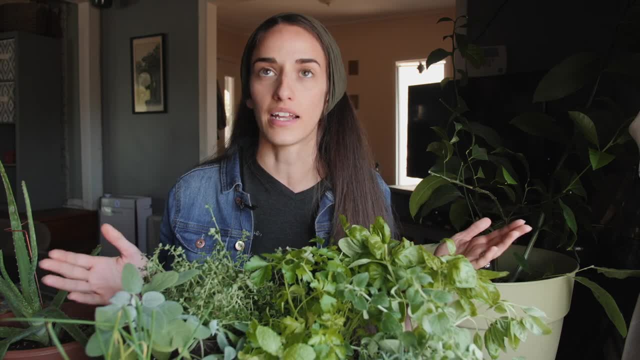 I tend to find that basil- though I love it and there are so many different types of it. The basil with the purple leaves is a little bit more tolerant, but it's a very, very good choice, And then just that one. I tend to find basil is probably the best thing to use in the summer because 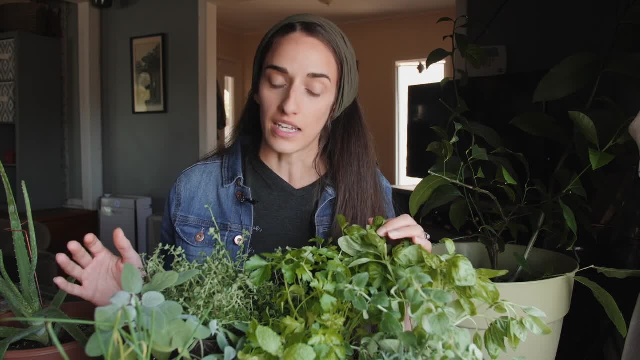 it's a little bit more tolerable, but it can be a lot more very hotel-friendly. So if you're in the country and you want a more urban climate, this is a good time to go to your mill. a lot of different leaves is a little bit hardier, Basil's finicky. I kind of call it a princess herb. It needs to be. 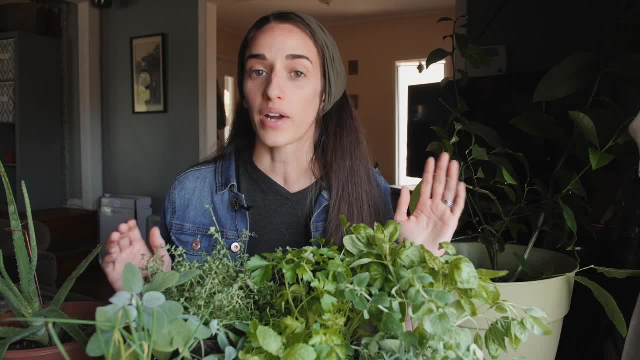 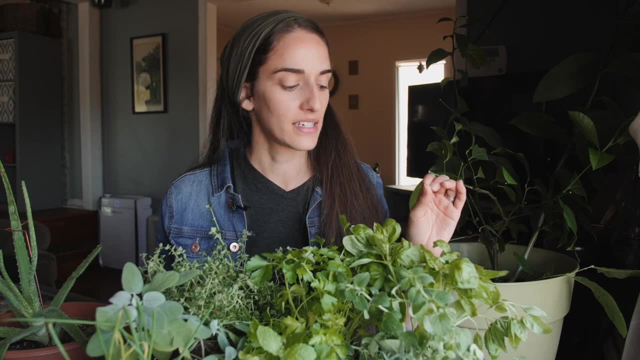 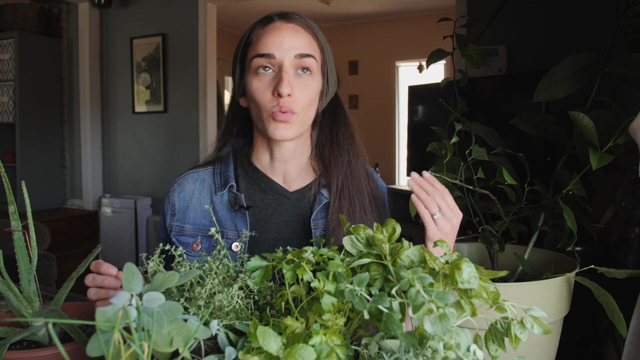 catered to a little bit more than the other herbs. So I highly recommend giving it a go, because it's amazing to put in so many things. But it can be a little bit tricky, as it likes a very specific amount of water and a very specific type of soil. And the last one that some people really don't: 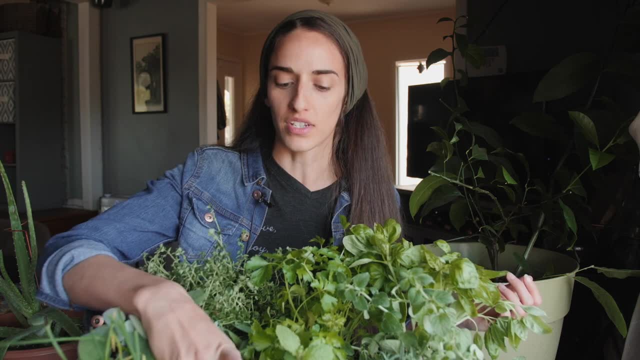 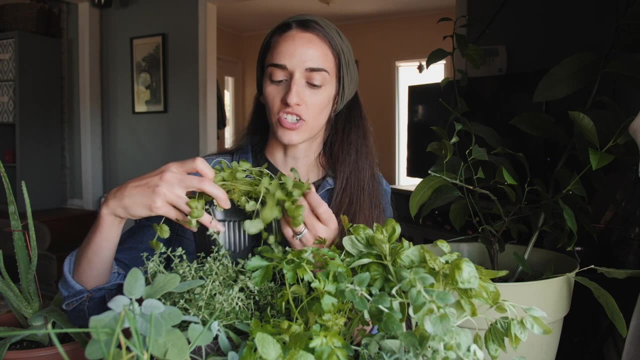 like at all and some people love is cilantro. I'm just going to pick this one up because it's drooping in the front. I am one of those type of people that love cilantro. Some people, like my mama- she cannot stand cilantro. But cilantro again, it's an annual herb, just like basil. 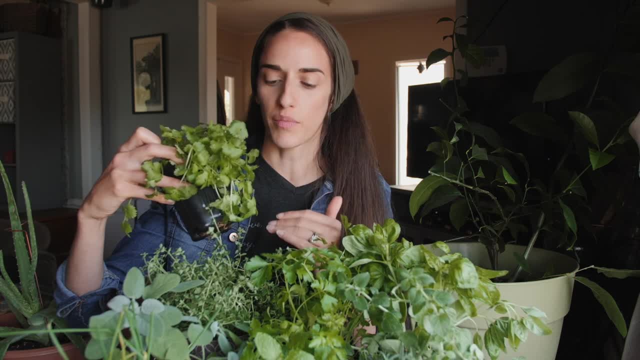 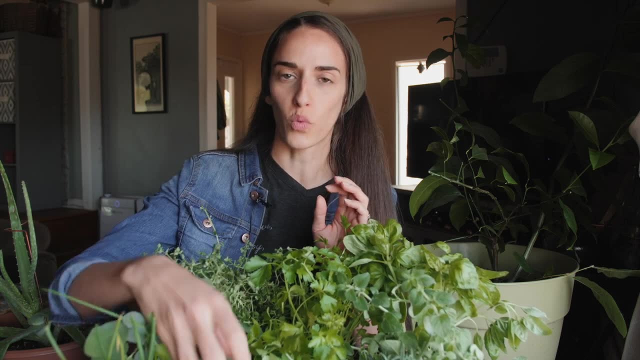 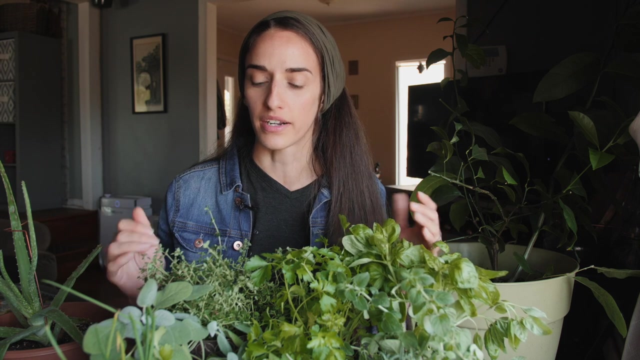 And cilantro, I believe, will self-seed. I will put this information for you, by the way, in the comment section pinned below. It's a little bit of a princess herb as well, but worth giving a go. So to recap here, if you are just starting out and you are going to have a small space, herb garden: 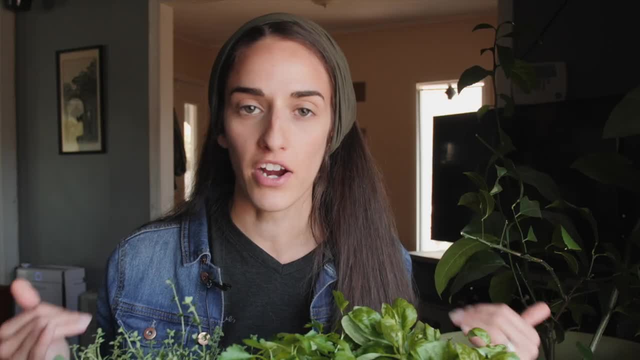 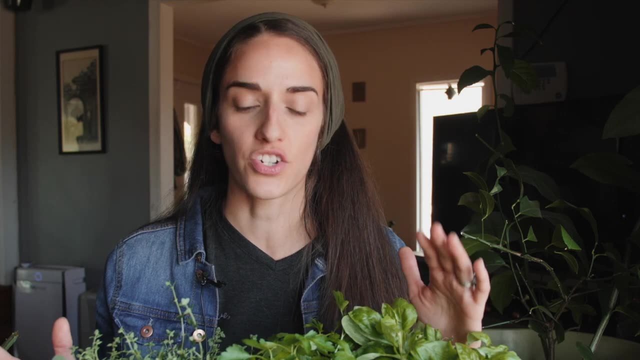 and get your feet wet in terms of growing plants. in my very humble opinion, I would start off with your thyme, a mint or a lemon balm, your oregano and your rosemary, And you can grow them in a windowsill. 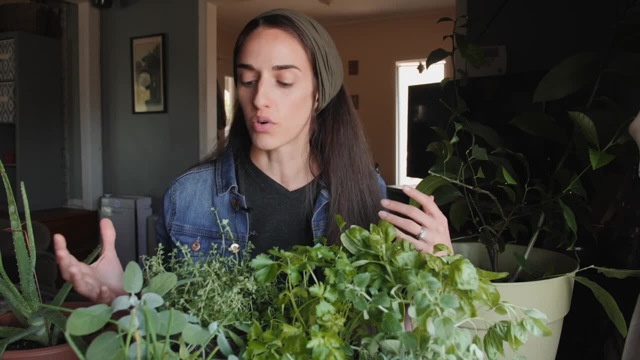 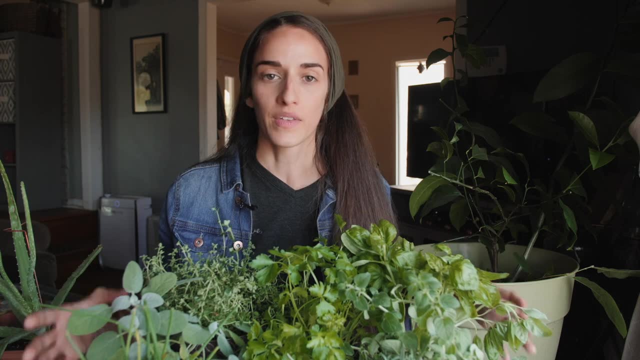 you could grow them outside, you can grow them in pots, you can grow them in the ground. Even if you live in an apartment and you only have one sunny window and you have no balcony outside, get yourself a little plant stand with different levels by that window and just some pots. 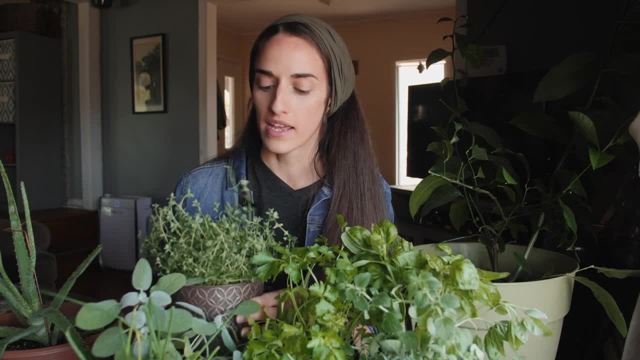 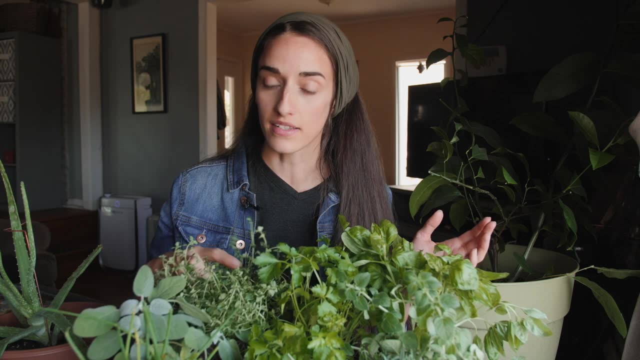 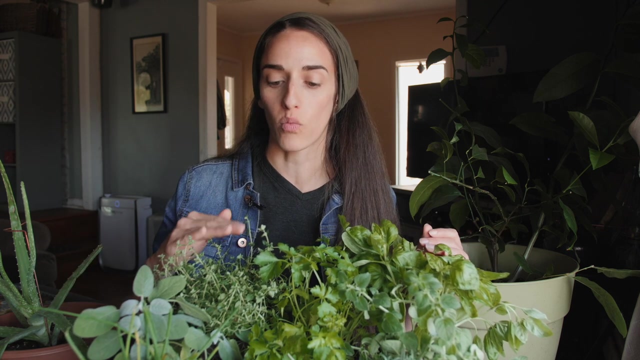 Sometimes you can even thrift pots Or people are giving them away. Get yourself some really good organic potting soil and then either plant baby plants that somebody gives you or you find at the store or plant them from seed. If you're planting them from seed, begin out by watering them, by spraying them every day. 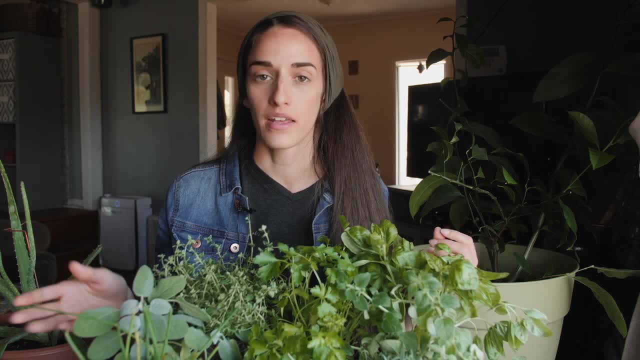 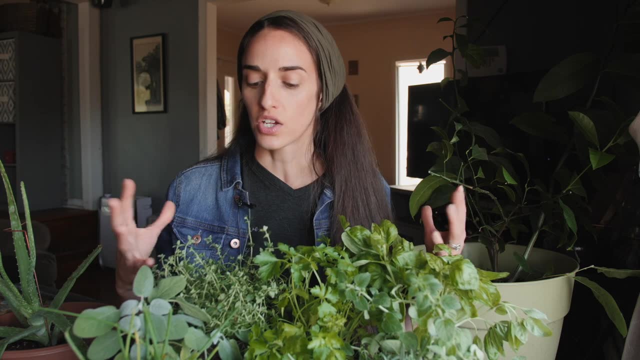 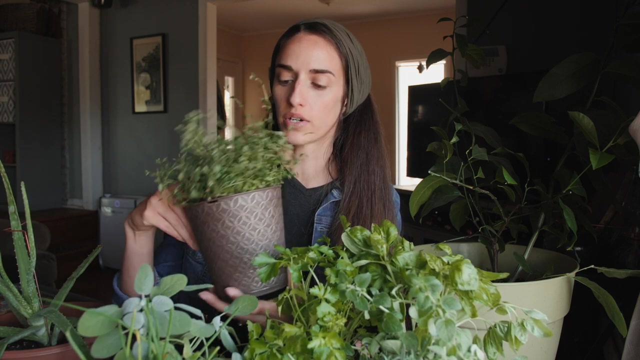 twice a day. You don't want the soil to get too wet or the seeds will rot, but you also don't want them to get dry. And then, as the plant grows and matures and gets stronger roots, you can water them once a day or whenever the soil doesn't feel moist. So you push your finger down into your soil. 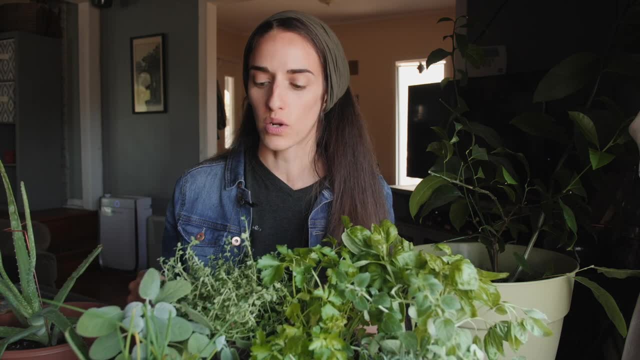 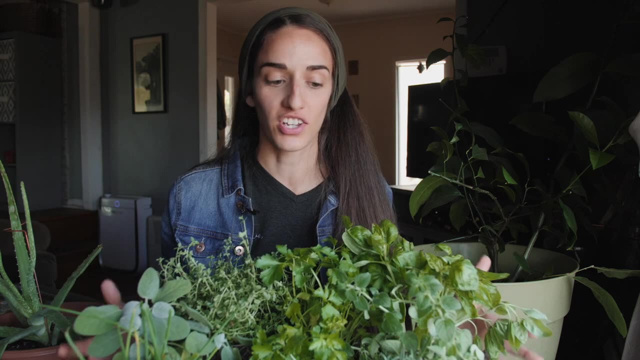 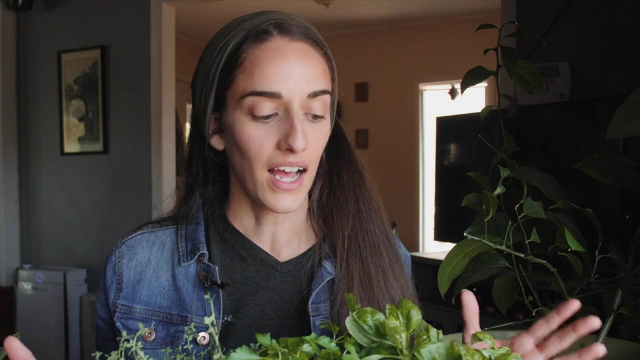 about two inches, and if it feels dry, give it a little bit of water, but not too much. Sometimes people over-nurture their plants and they give them a little bit too much of the good stuff. So balance in everything and don't fret if it doesn't work out. You can always begin again. 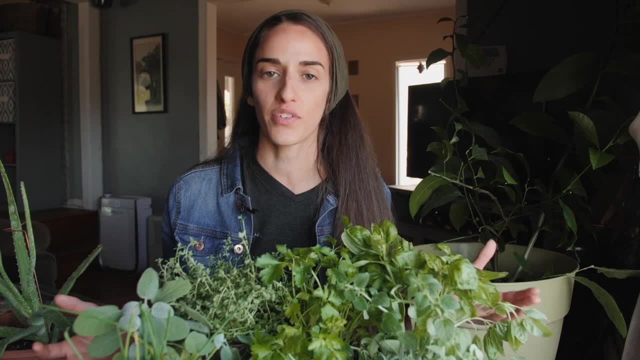 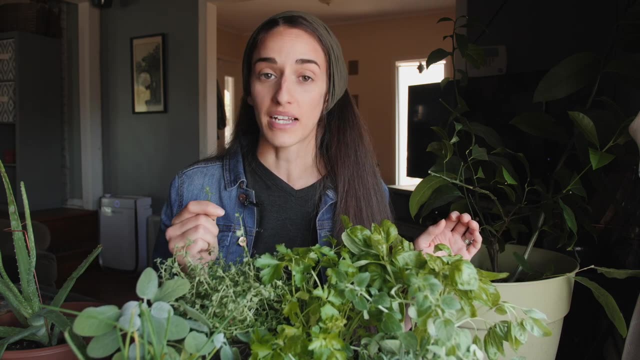 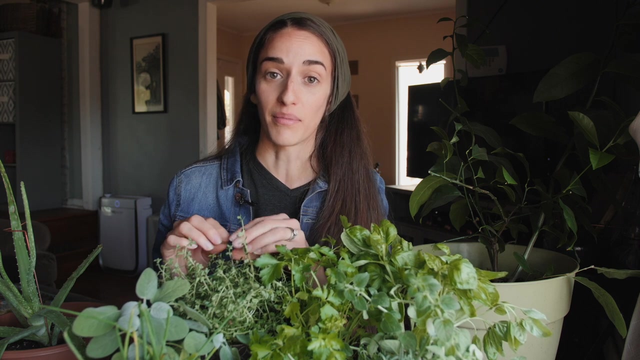 I hope that this was some good information for those of you again who just want to get your feet wet. get started in growing all the green things And I'm telling you, be careful, because when you start growing all the green things, you're going to want to grow more of the green things, And then it becomes a thing. 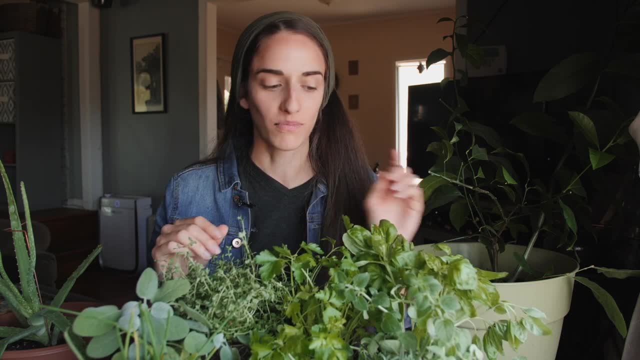 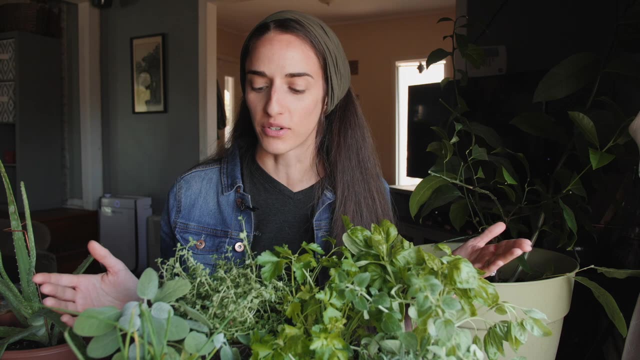 That's really good. I'm just going to excuse me, And you know what. You can make an entire salad just out of herbs and it's so good for you. All right, friends. Well, if you are going to give this a shot this year, 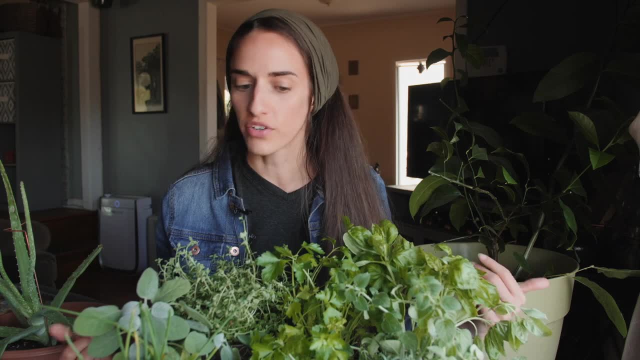 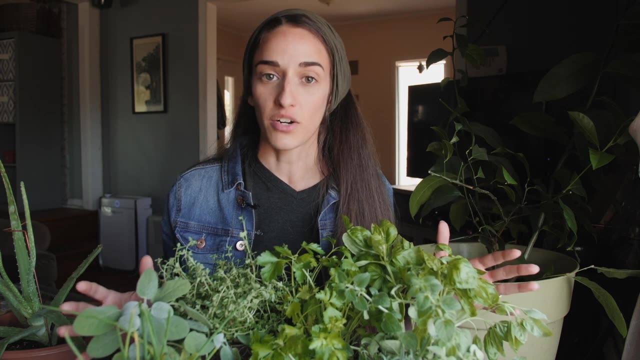 put it in the comments below. Let me know what you're thinking about doing. Where are you going to be planting Balcony windowsill indoor, outdoor? Let me know what you're going to venture into. I would love to hear about your plans And I wanted to say thank you so much as always for 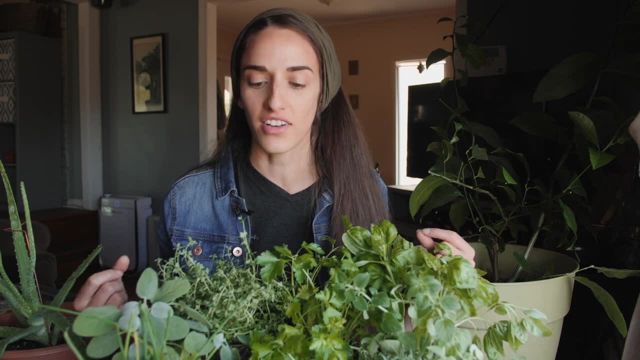 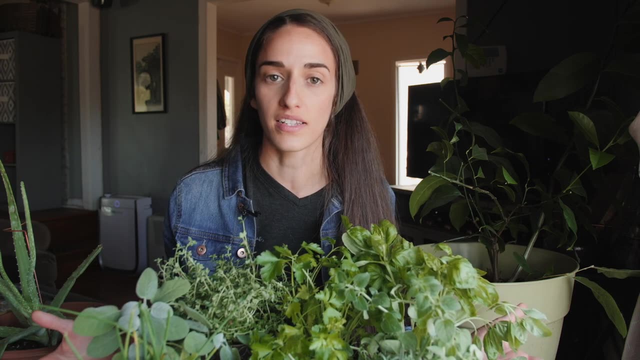 coming back to our little house in the mountain. If you have any questions or comments, please leave them for us. Let us know if there are any videos that you want to see. We're so thankful to you and thank you to all of you for joining us today. We'll see you next time. Bye-bye. 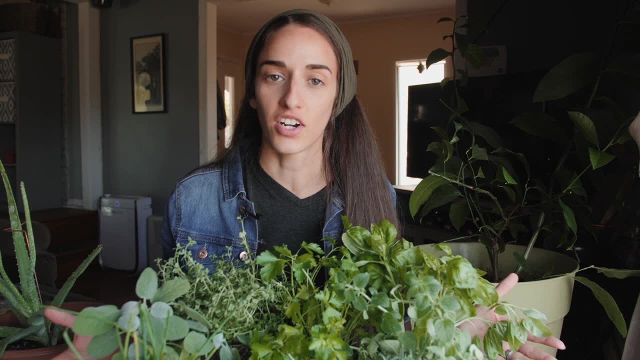 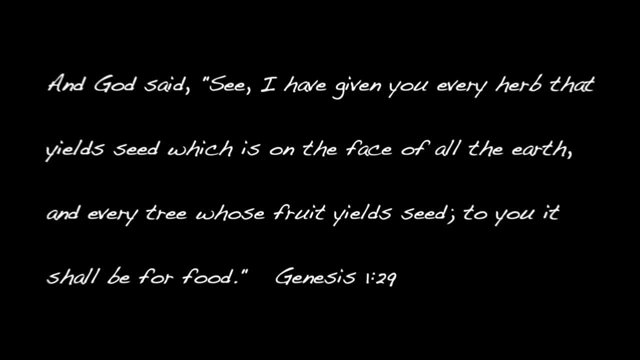 Thank you to our patrons over on Patreon for supporting the content here. We love you guys with all our hearts. Happy growing, and I'll see you on the next one. Shalom to your home, Bye.